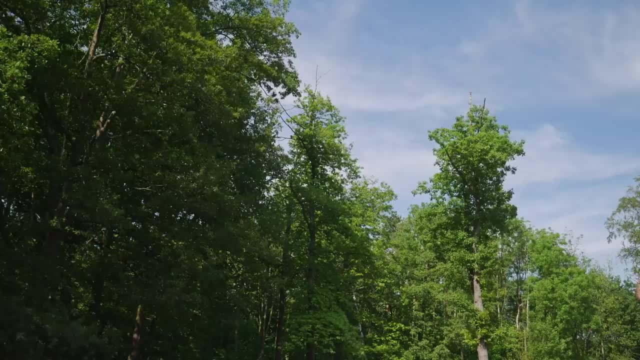 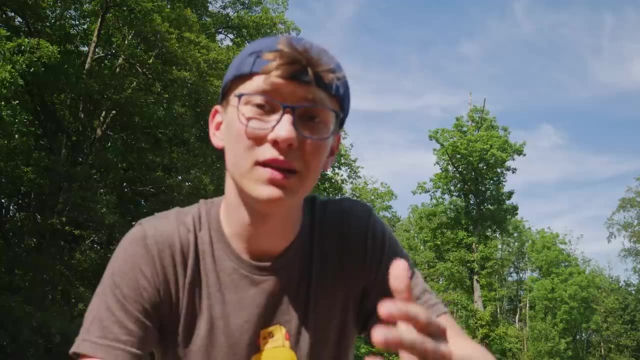 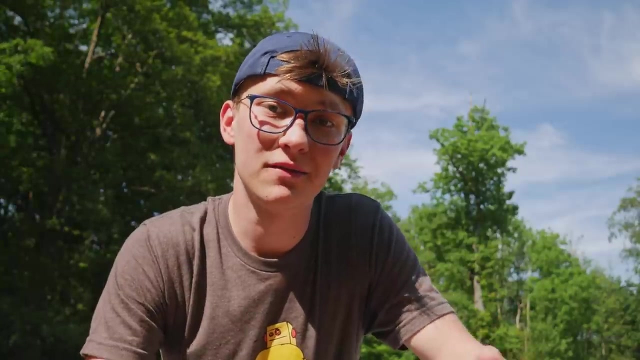 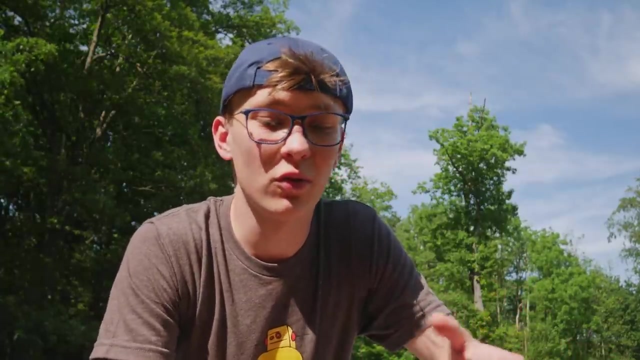 I started with robotics by playing with Lego bricks and I know that's not really robotics, but when I was about 6 years old that was a great way for me to build anything I wanted And it also broadened my imagination. you know it was very creative. Later I got the power functions kit- that was a motor with batteries, so that you could create stuff out of Lego that is moving. you know cars, robots, machines. 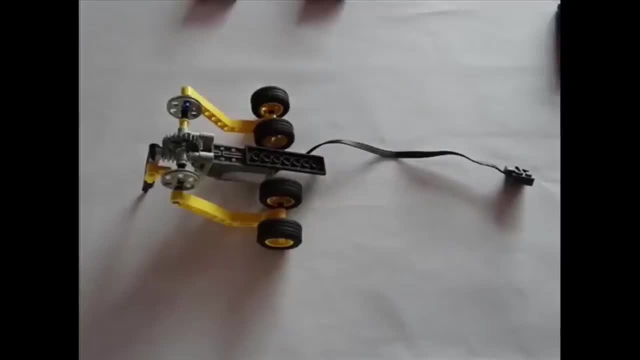 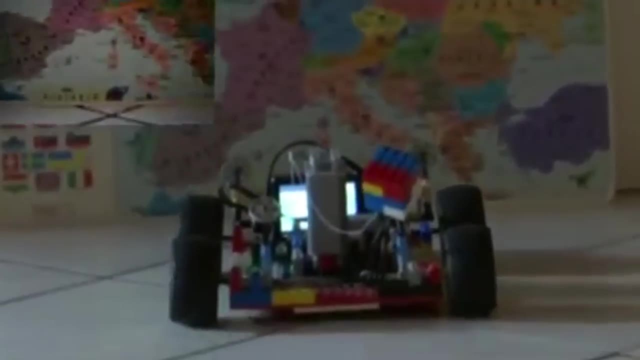 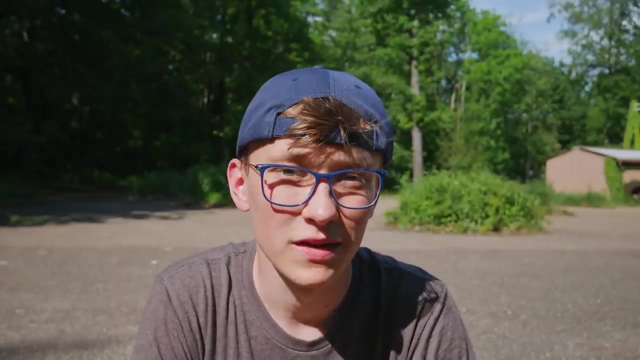 So I started building basically that- cars, robots and machines- And I also started making my YouTube videos. My first- I think 3- YouTube videos were about Lego constructions. you can still see them on my channel. When I was about 12 or 13,, together with my dad, we built first real robot with electronic components, some cardboard and motors that I took out of old toys. 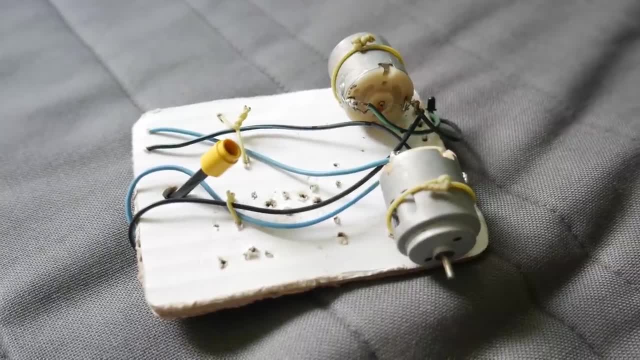 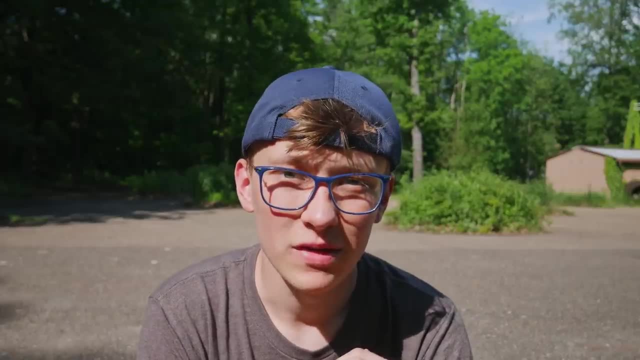 Those motors were attached to the cardboard with piece of wire. This build was really crappy. like the engineering side of this project was terrible, but it was kind of working. It was a light following robot and there was nothing to do with it. So I started making my first robots and I also started making my YouTube videos. My first- I think 3- YouTube videos were about Lego constructions. you can still see them on my channel. 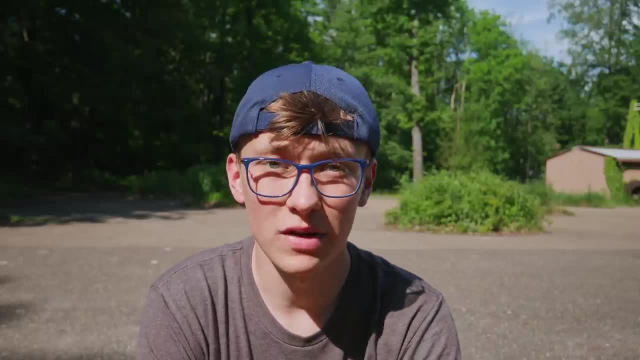 And I also started making my first robots and there was nothing to do with it. So I started making my first robots and I also started making my first Lego constructions. you can still see them on my channel- And there was no programming involved. This kind of robotics where there is no programming is called BIM, which stands for Biology, Electronics, Aesthetics and Mechanics. 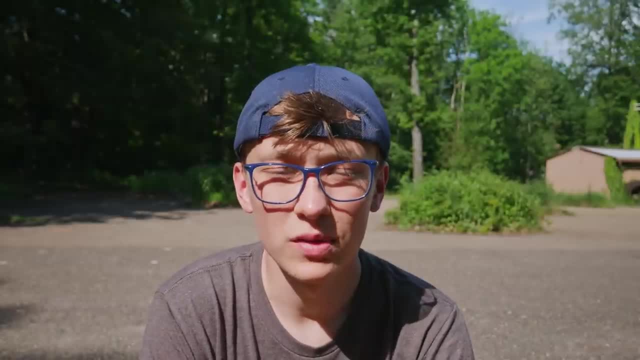 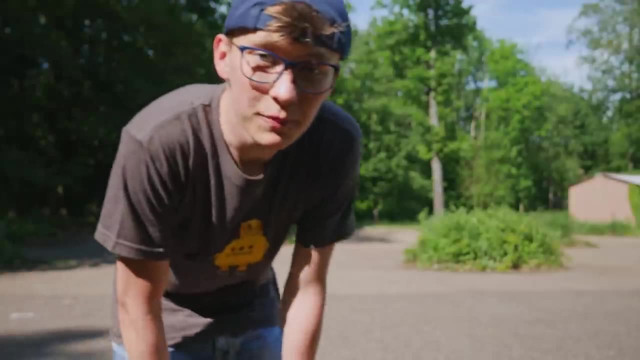 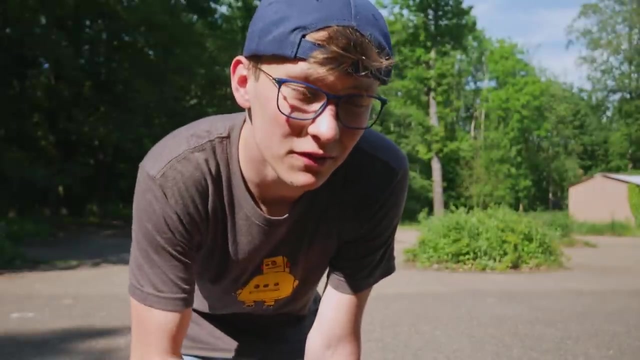 It's a really cool way to start with robotics, to learn and to build simple stuff, but to build something complicated and big, it's plain ideas to use just analog circuits. In April of 2014,, I've got my first Arduino. I remember this day exactly And because at that time I already had quite a lot of experience with programming, it was super easy for me to learn how to program. 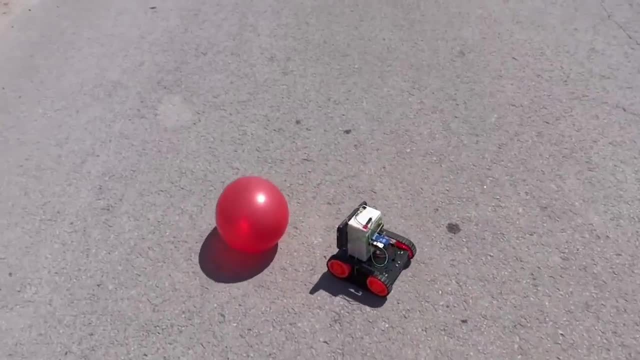 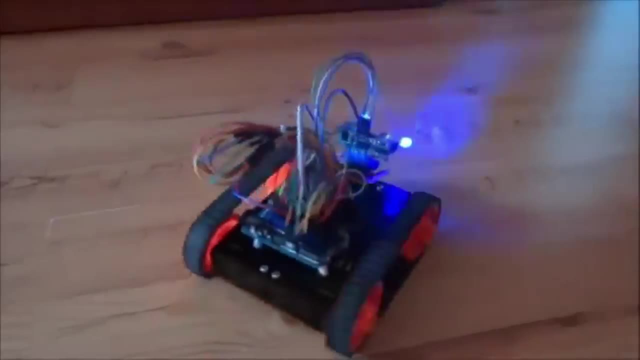 In April of 2014,, I've got my first Arduino. I remember this day exactly And because at that time I already had quite a lot of experience with programming, it was super easy for me to learn how to program, So I started putting out a lot of different projects- robots, machines. you can see most of them on the instructional boards or here on my YouTube channel. 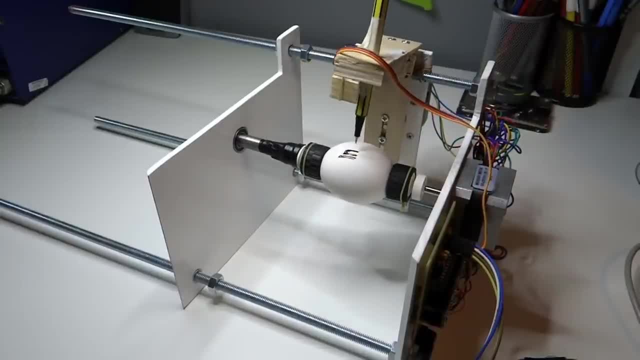 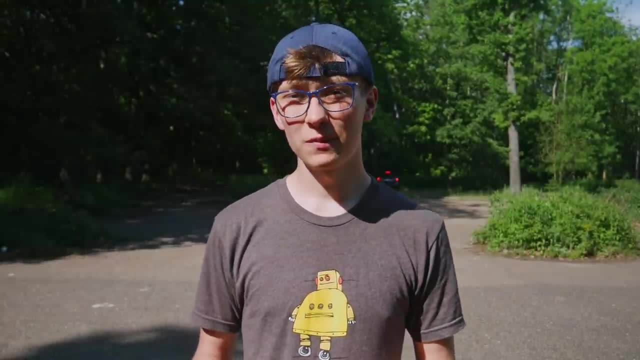 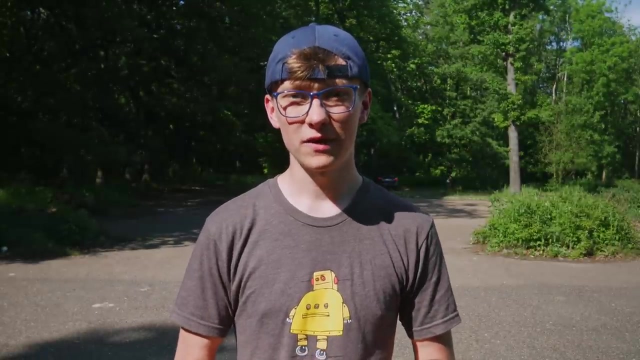 If you have any visual functions that are arriveing in the future, please share. Now' it's 2019,. I'm already 5 years into making this kind of projects and robots. I have a little bit of experience with industrial solutions, but I really don't like those overpriced, closed environments developed by companies that are afraid. 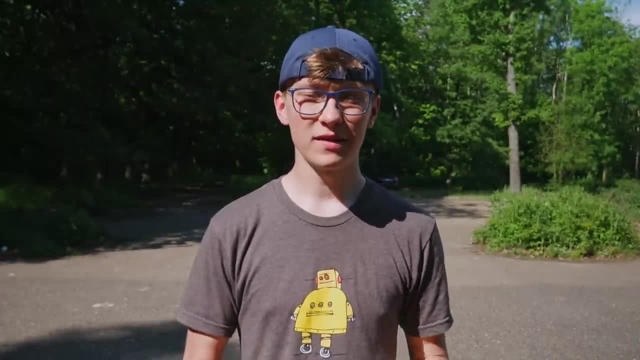 I have a little bit of experience with industrial solutions, but I really don't like those overpriced closed environments developed by companies that are afraid develop new technologies. What I like is open source, inexpensive and easy to use. What is inexpensive and easy to use- LCSC electronics, So let's jump to the 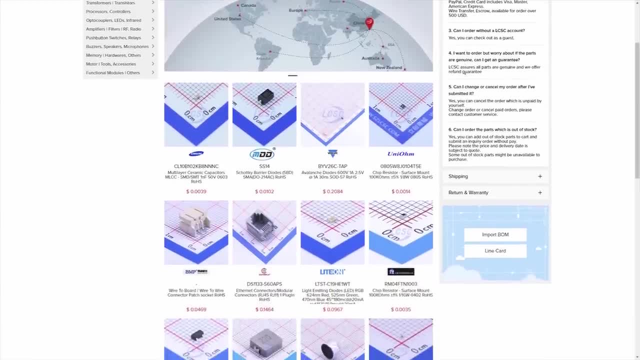 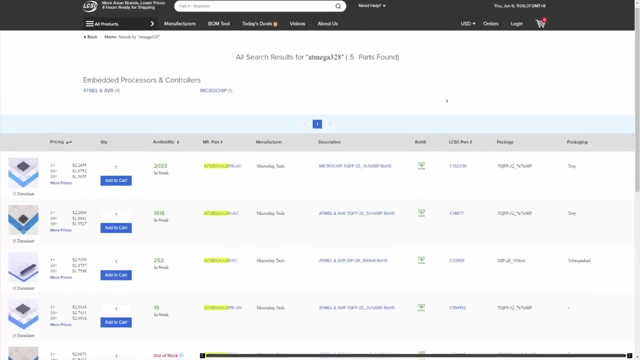 sponsor message. Sponsor of this video is LCSC electronics online store with electronic components. You can find the rare components that are hard to buy anywhere else, but also as popular components as ATMEGA328 that you can use for your next robotic project. It's also a great place to buy components if 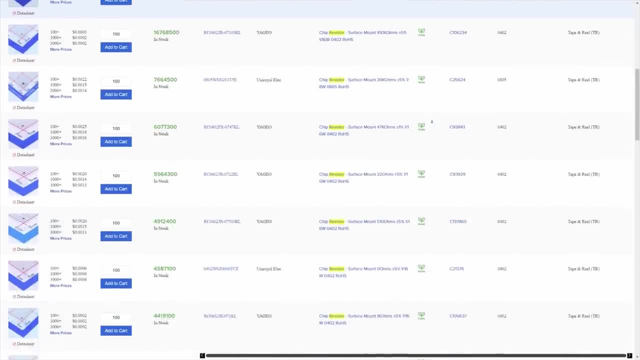 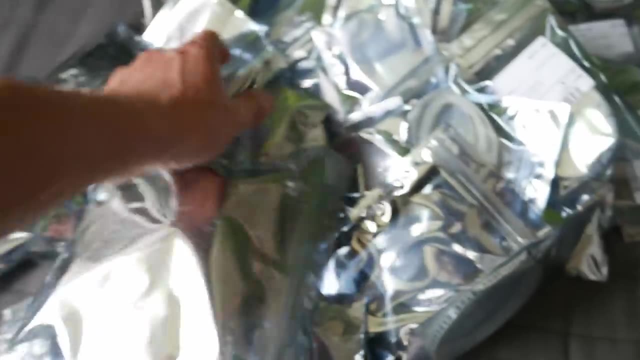 you want to start manufacturing your project. They have discount prices if you buy more. they pack everything really nicely and every component is labeled. I tested that myself. I will put a link to LCSC in the description. Go check it out. Maybe you will find here components for your next. 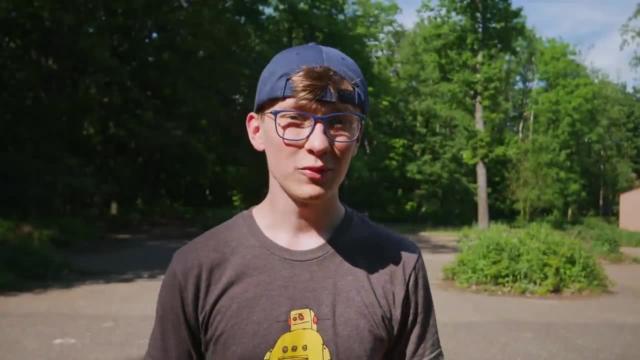 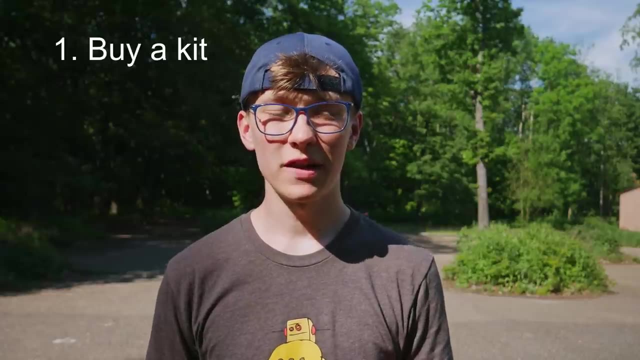 project. And now I will try to answer really not a simple question: How to start with robotics. Robotics is a really broad topic, so there is a lot of different ways how you can start with robotics. You can buy a simple kit online for few bucks with everything you need to build a robot. You can assemble that. 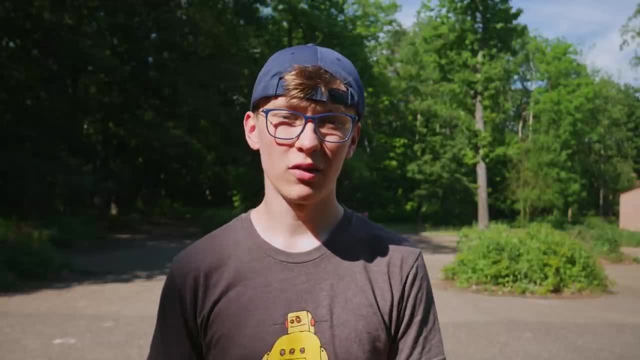 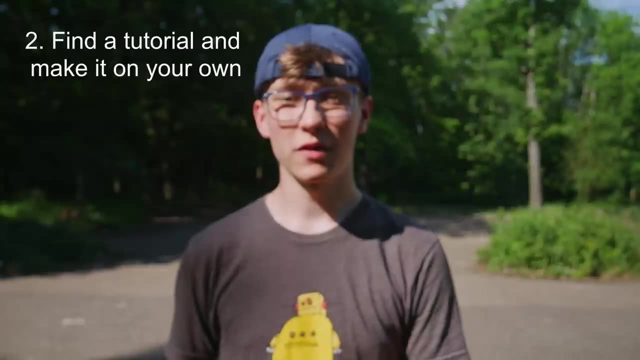 solder everything and you have a working robot. You wouldn't learn a lot by this- by soldering- But at least you can practice soldering and get to know all the components. Better way is to find the tutorial online on how to build some. 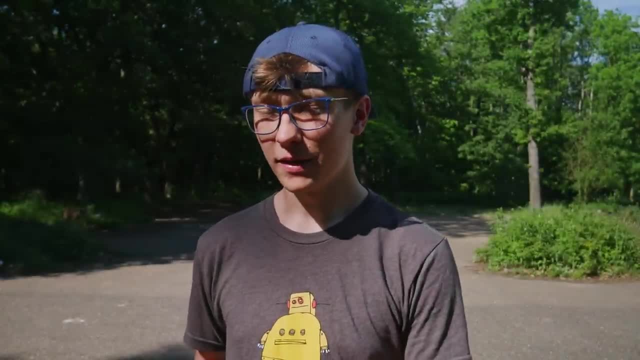 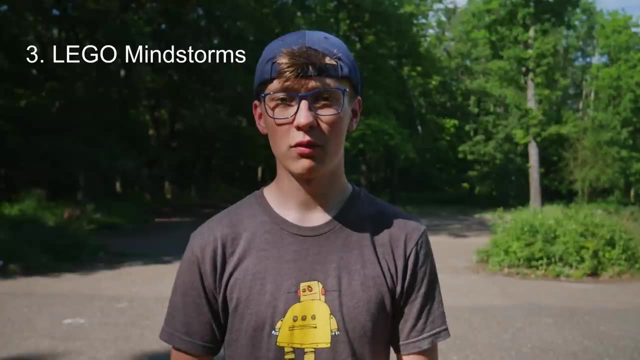 kind of beam robot, for example, light following robot, like I did, Buy all of the components by yourself and figure out how to assemble all of that to get it working. If you are young, maybe Lego Mindstorms is a way to go. Visual programming language is super easy to understand for kids and if you want to, 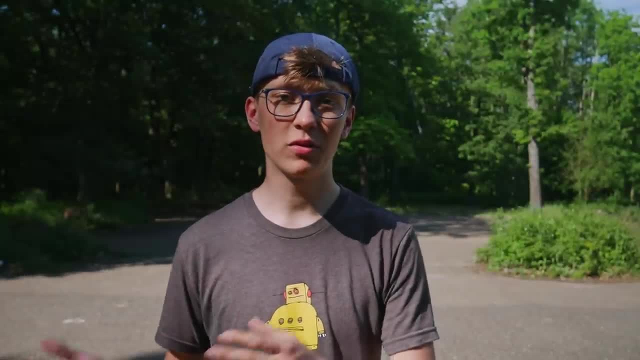 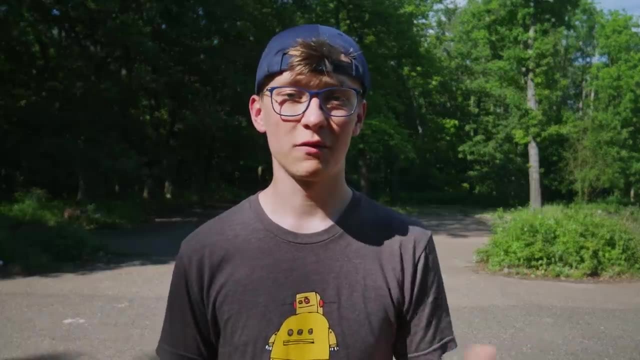 do more advanced stuff. you can do it with Java or C++. You can program the Lego Mindstorms with Java or C++ and because you know that's Lego that's simple to build, You don't have to worry about. I don't know- 3D printing, maybe CNC. 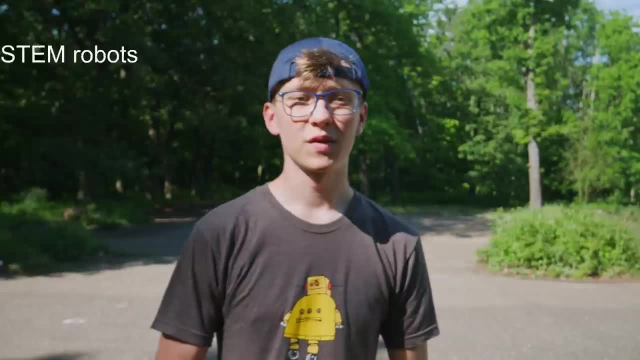 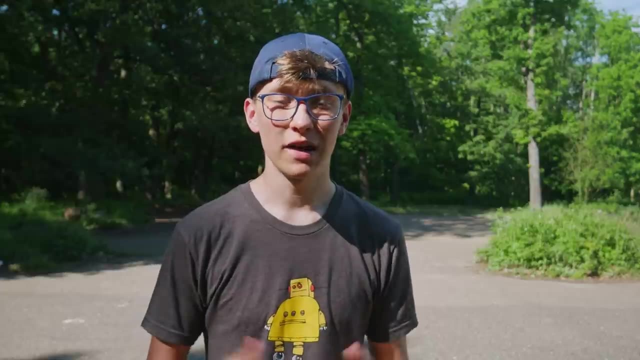 machining some of the parts. Everything is simple to build. There are also those STEM robots. however, it is called all over Kickstarter and Indiegogo. In my opinion, it's really not a good solution. Lego Mindstorms is definitely way better, because those STEM robots- you only can program them. There is no construction at 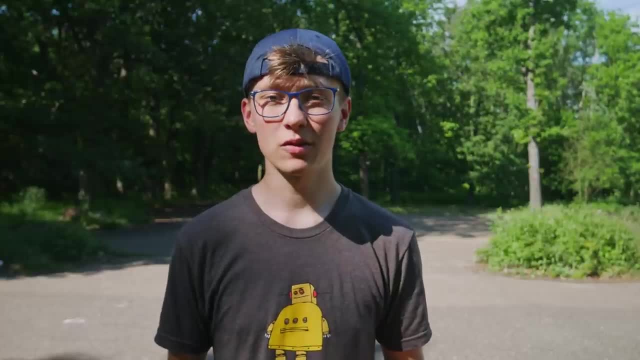 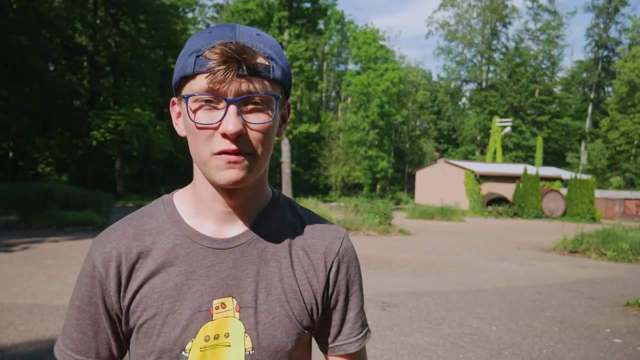 all. usually There are some exceptions. That's just too easy. Lego Mindstorms: let you construct stuff and you are not only limited to programming. That's a good thing, And here is, in my opinion, the best way to start with robotics: Just buy an. 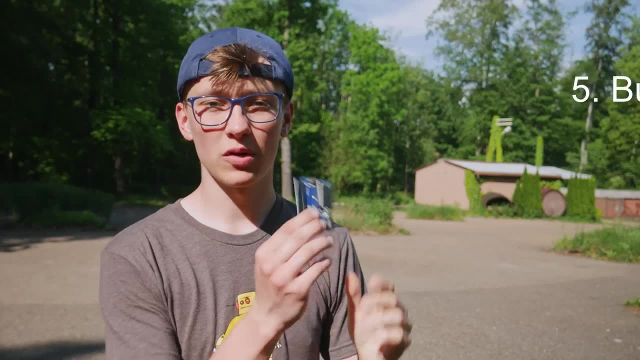 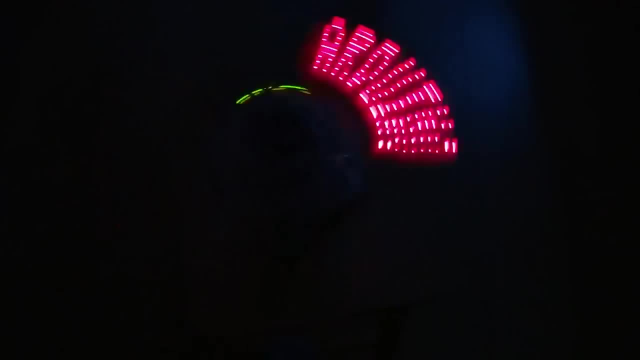 Arduino. It's inexpensive, easy to use. You can easily learn how to code with that. You can buy a lot of different sensors. learn to use them. build few projects like a weather station, an alarm clock or POV display, as I did Then you.